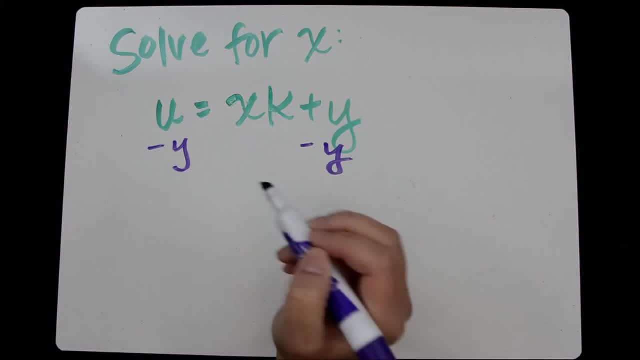 So we're going to subtract y from both sides of our equation. Here it zeroes out, and on the side we're left with u minus y is equal to xk, And then to get x by itself we have to undo the multiplication to k. so we're going to 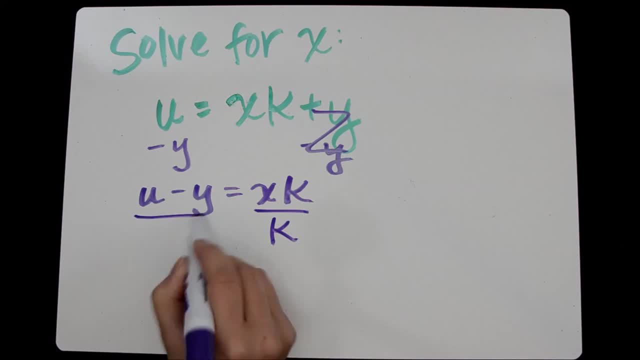 undo the multiplication by dividing both sides by k, And when we do that, this one's out. we're left with. x is equal to- and I'm just going to rewrite it on the left hand side- u minus y, all over k, And that is our simplified answer. We can't combine any of the variables because they're. 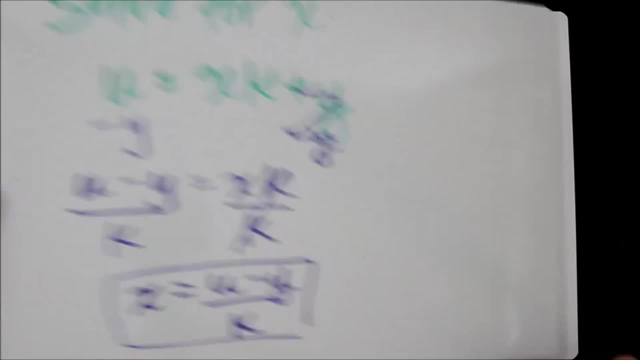 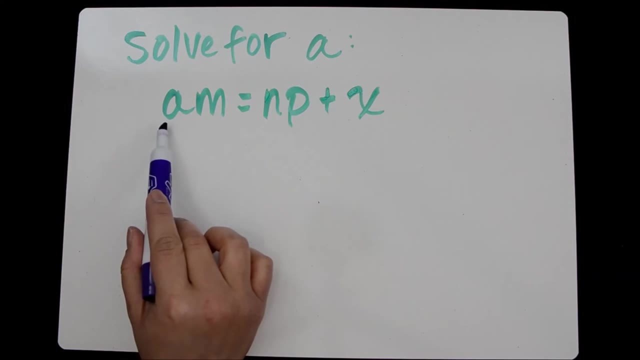 not like terms. Let's take a look at our next example. This problem is asking us to solve for a, and so we're trying to get a by itself. The only thing keeping it from being by itself is the multiplication to m. So, to undo the multiplication, we're going to divide. 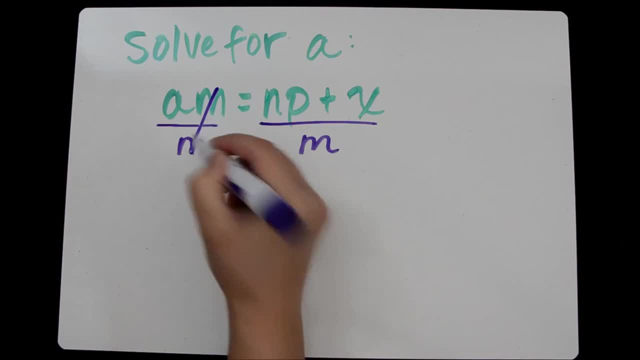 and whenever we divide, we divide everything. So here it ones out and we're left with: a is equal to np plus x all over m. Again, none of these terms can be combined because they're not like terms. Let's go ahead and take a look at an example with some numbers. So here they're, asking us to solve. 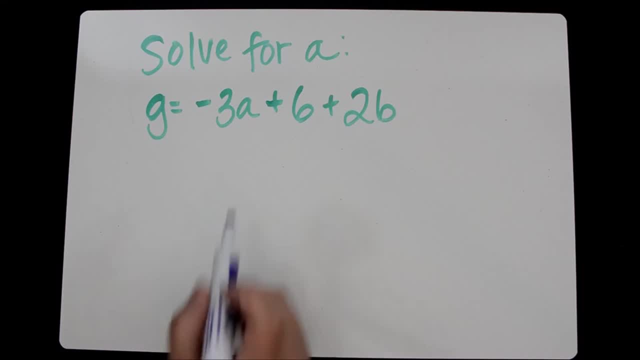 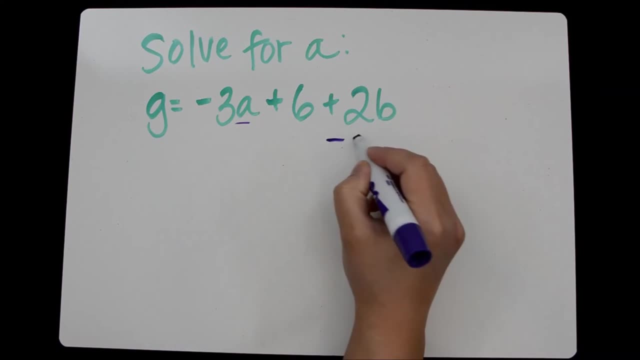 for a, and it doesn't really matter which order we're going to undo the addition terms, So I'm just going to start with a. 2b. I'm going to subtract 2b from both sides of our equation and I'm going to write this in alphabetical order. So I'm going to rewrite this as negative 2b. 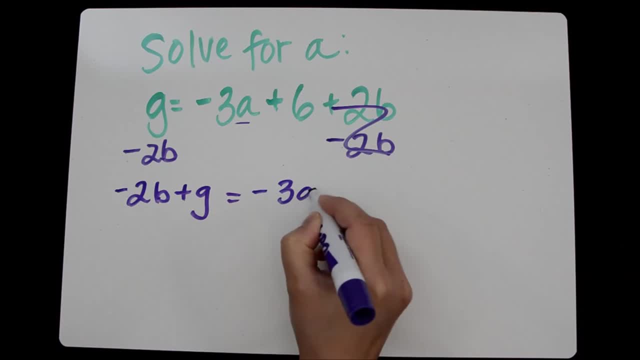 plus g is equal to negative 3a plus 6.. And then now I'm going to undo the constant, I'm going to subtract 6 from both sides. The 0 is out and we're left with negative 2b plus g minus 6 is equal to. 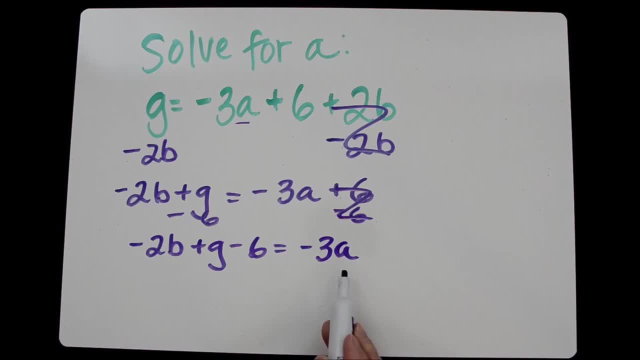 3a, And now the only thing I have to undo is the multiplication. So I'm going to divide by negative 3 and it ones out here. So I'm going to rewrite this, correcting some of the signs or simplifying some of the signs. Negative 2b over negative 3 would become positive 2b and then